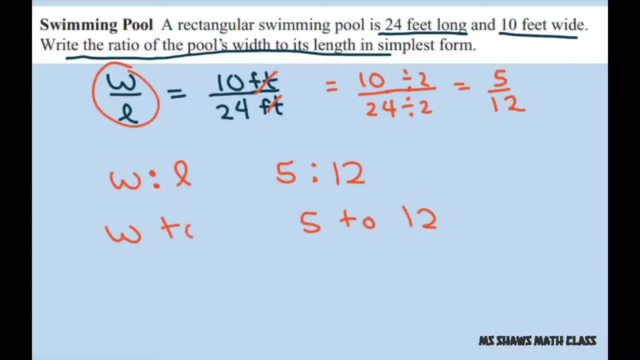 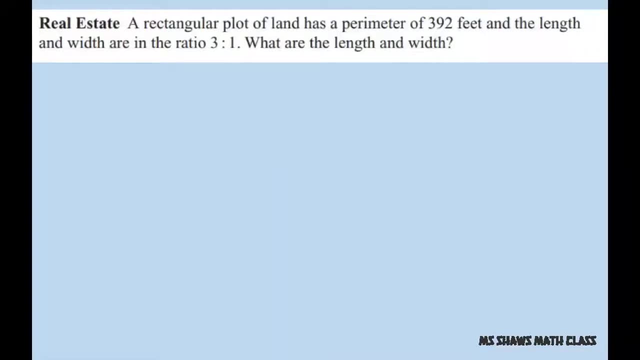 if it said width to length, All right. now the next one. it says a rectangular plot of land has a perimeter of 392 feet and a length and width are in a ratio of 3 to 1. So we're talking about perimeter, and that's: 2L plus 2W equals your perimeter. Well, my length. 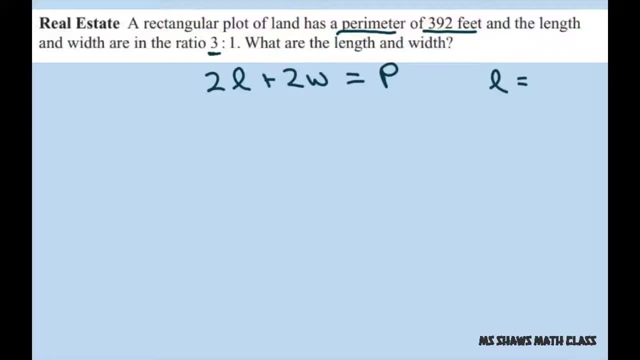 I'm going to call 3X, because that's the ratio of 3 to 1, and my width is going to be 1X, which is just X. So now what I'm going to do is substitute this in, along with my feet here. 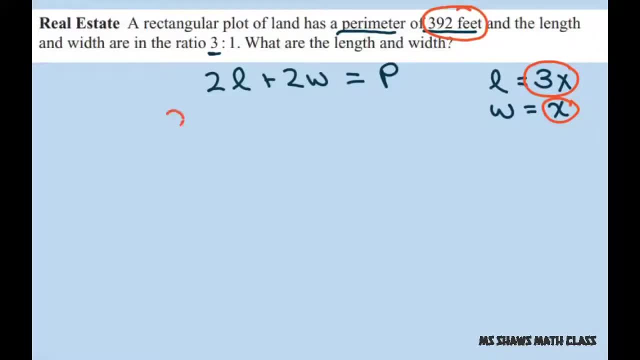 And we'll solve for X and then find the length and width. So the length is 3X, The width is just X and the perimeter is 392 feet. We'll leave the feet off for now. So this is going to be 6X plus 2X equals 392.. 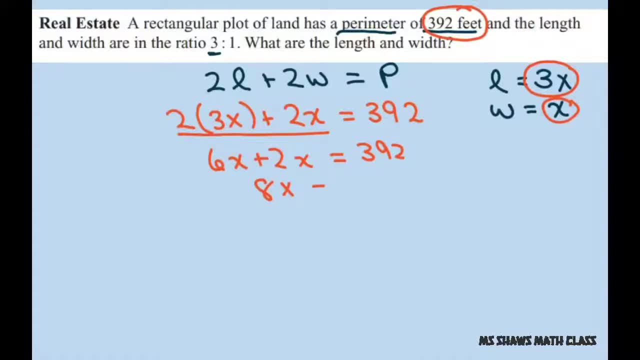 So 8X equals 392.. And divide both sides by 8. So 8 goes into 39 four times with 7 left over. So you have 72 and 8 goes into that 9.. So X is 49.. And you can multiply it back and check, But that's doing it without a 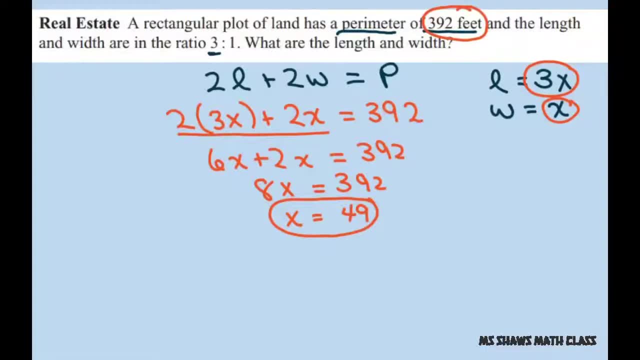 calculator. Now we're going to find the length and width. So the length is going to be 3 times 49. And that gives you 3 times 50 is 150 minus 3. It's going to be 147. And that's going to be feet, And the width is just going to be X, which is 49, and then feet. 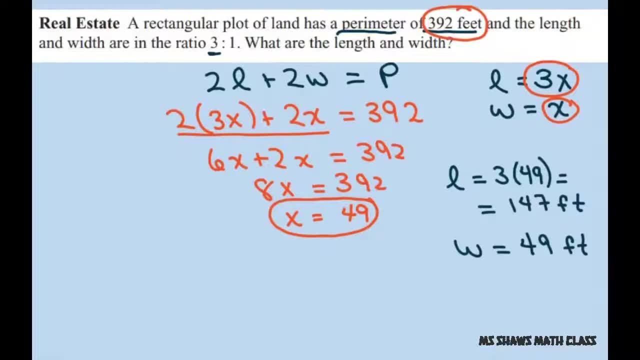 And you can always check your answer by plugging it in. So we can do: 2 times 147 plus 2 times 49 should equal 392.. So 2 times 147 is going to be 1492 plus 98. And that gives you 392.. So it checks out. 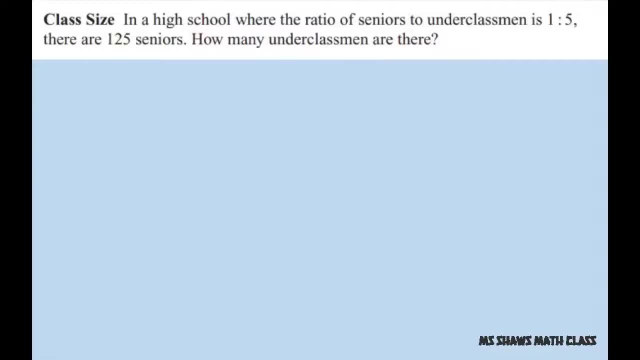 Okay, the class size In a high school where the ratio of seniors to underclassmen is 1 to 5. So seniors equals 1. And underclassmen- I'll just put under- is 5.. So keep it straight here. And we know there are 125 seniors. 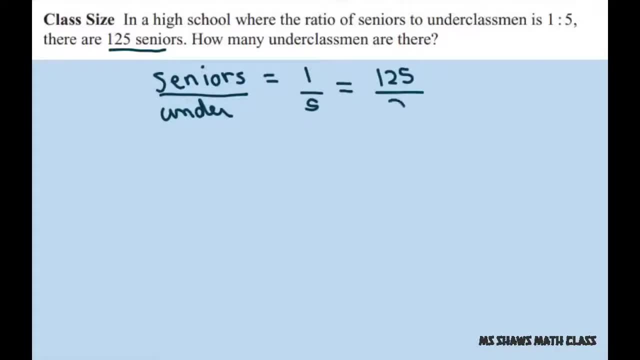 So how many underclassmen are there? So that's your unknown. So do you see how I kept my seniors in the numerator and my underclassmen ratios in the denominator? Now cross, multiply and you get X equals 5 times 125.. And that's going to give you, let's see, 5 times 125. 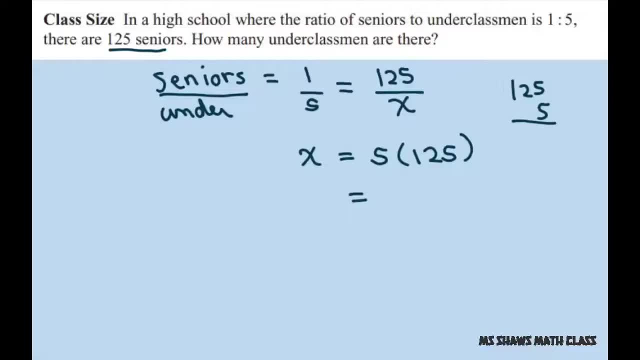 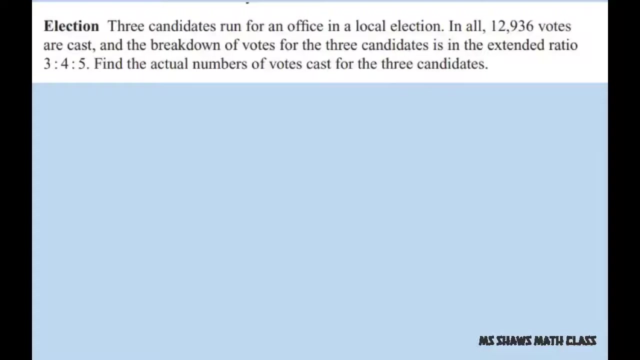 That's going to give you 4 times 125 is 500, so that's going to be 625.. So that's going to be how many underclassmen there are. And the last one says three candidates run for an office in a local election. 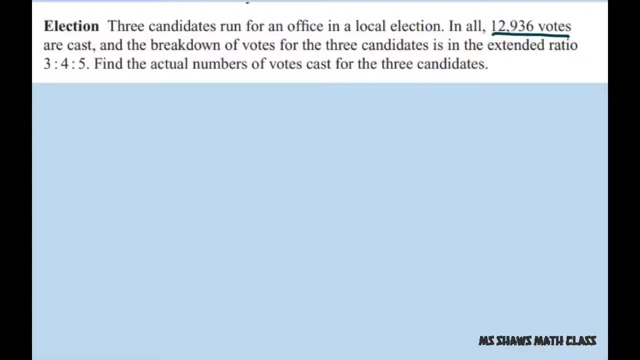 Here's your total votes. The breakdown of the votes for the three candidates is in the extended ratio of 3 to 4 to 5. There's three candidates. Find the actual number of votes cast for the three candidates. So what we're going to do.